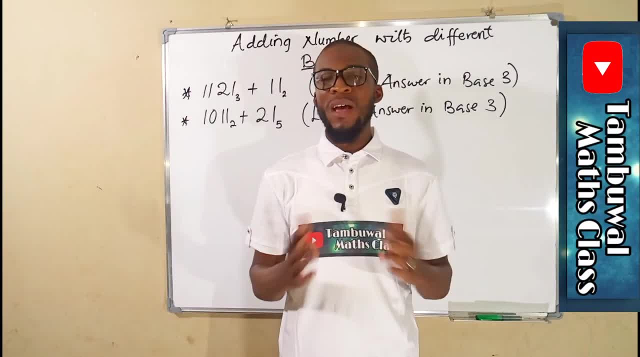 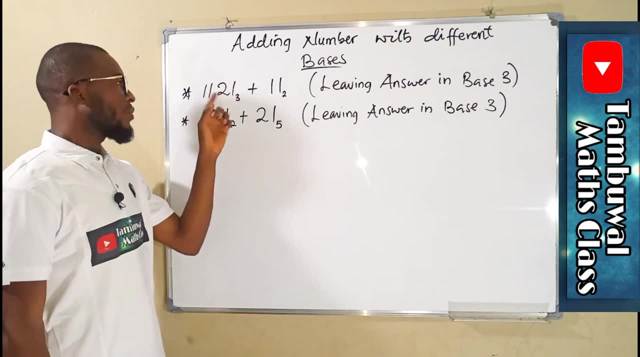 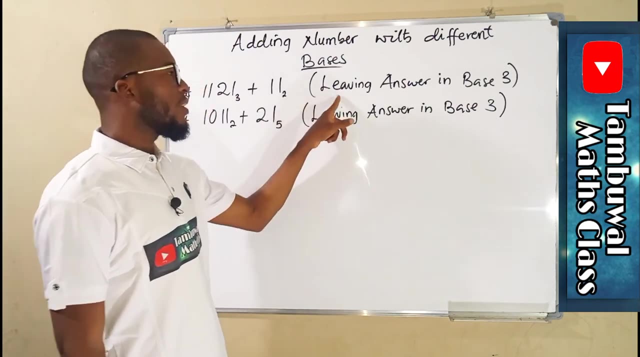 Into this tutorial. I will show you how to add numbers that are in different bases, And I have only two questions for today. The first question: we are asked to add 1121 in base 3 plus 11 in base 2, but it says we should leave the answer in base 3.. Since one of the 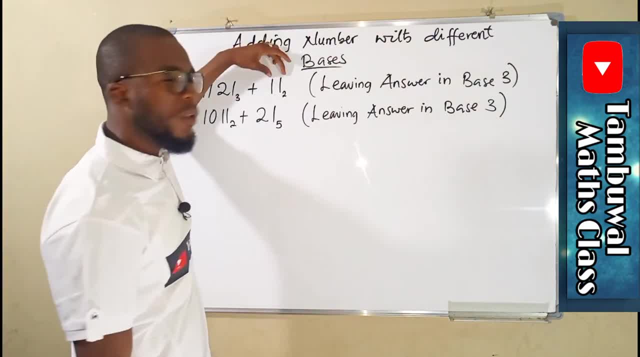 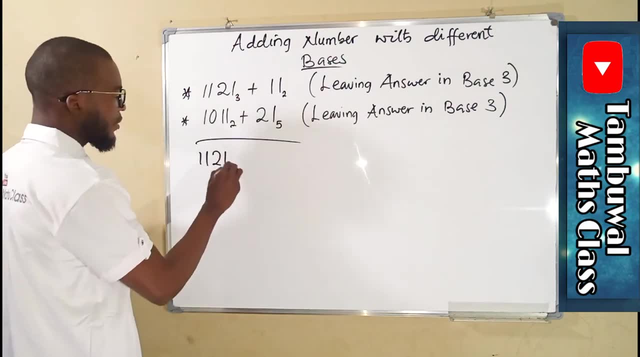 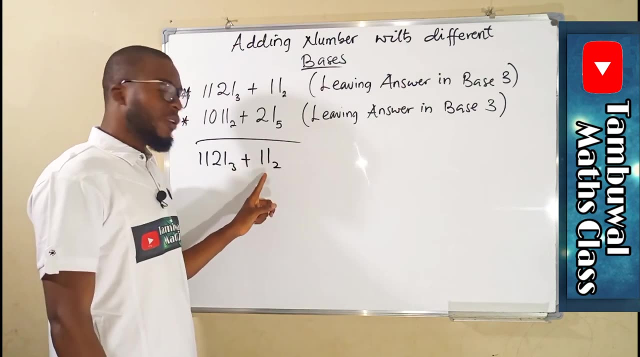 components is in base 3, we can just transform the other part to base 3, then we add them together and we are good to go. So we have to transform 11 in base 2 to base 3, we first of all have to convert it to base 10, then from base 10 back to base 3.. We have seen 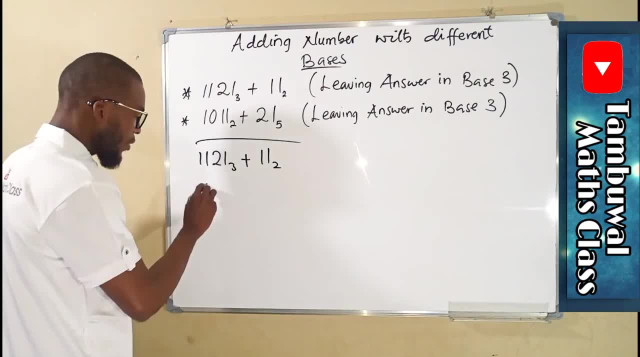 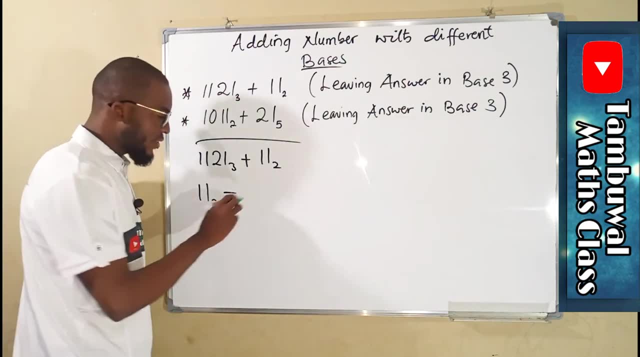 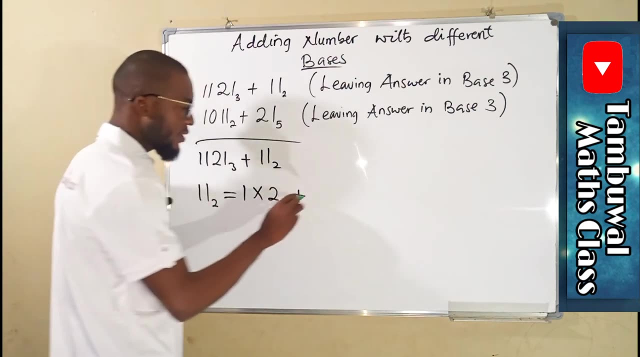 that in our previous lesson. So we have 11 base 2, we want to transform it into base 10 number. We take the first digit, 1. We multiply by the base, which is 2.. Then we add. We take the second digit, 1. We multiply. 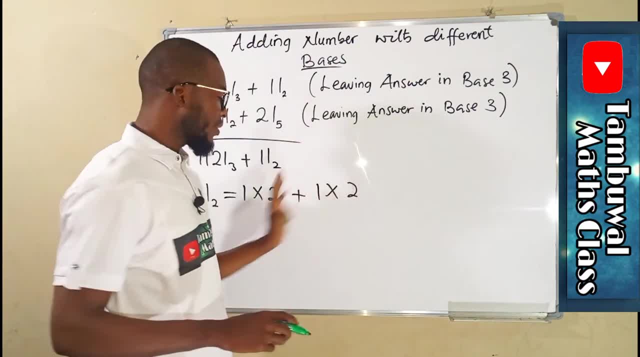 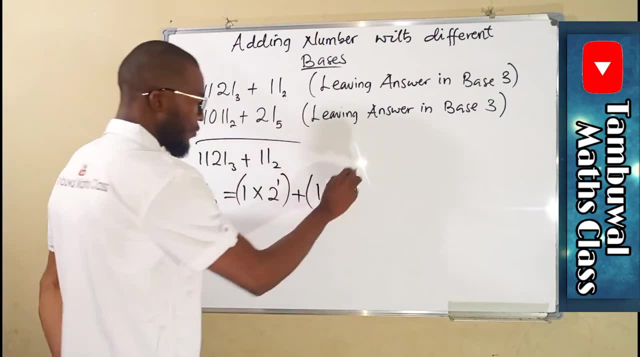 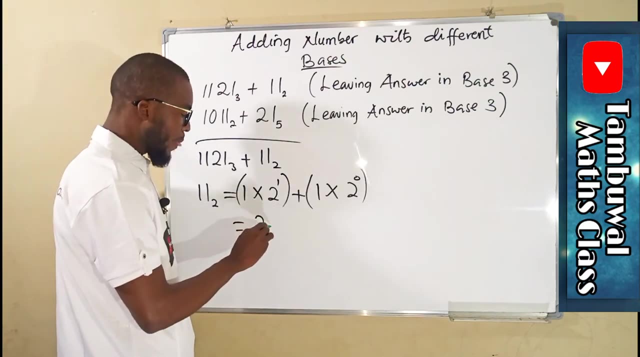 by the base. We assign our index from right to left, starting from 0, 1.. We stop. This is equal to 2. power 1 is 2, times 1 is also 2.. We have plus 2. power 0 is 1, then 1 times. 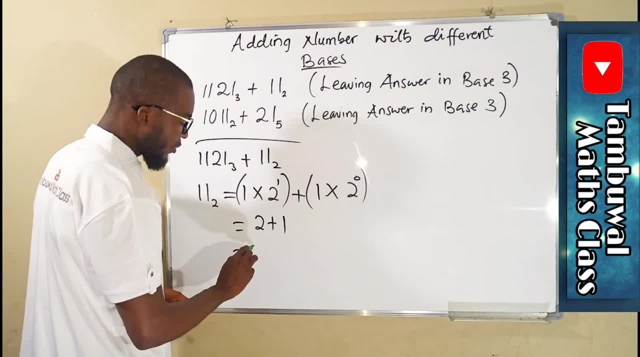 1 is 1.. We multiply by the base, which is 2.. Then we add, We take the second digit, 1.. And finally we have our answer to be equal to 3 in base 10.. Now we are free to. 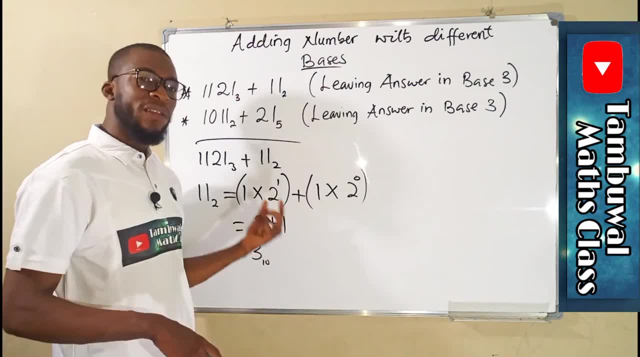 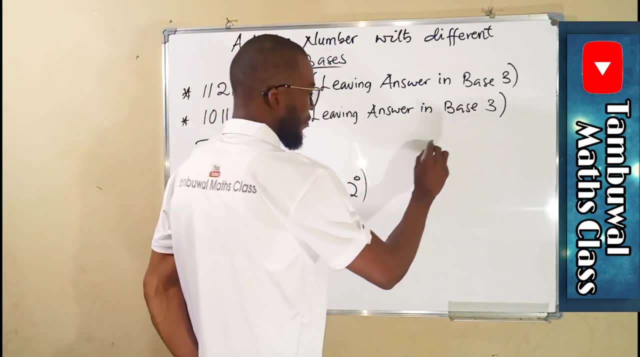 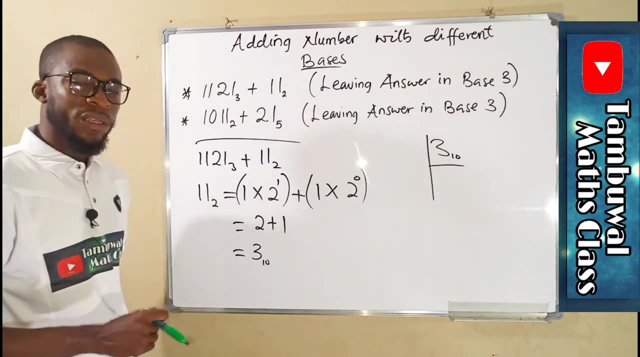 take this number, 3, which is in base 10, and convert it into base 3. in such a way, we are going to have a common base, So 3 in base 10.. We are going to form a successive division of this number using 3,, which is the required base. 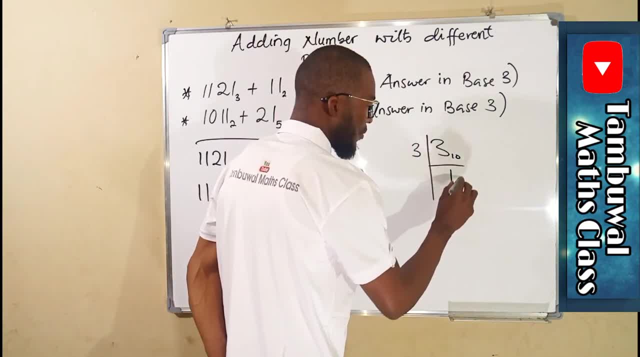 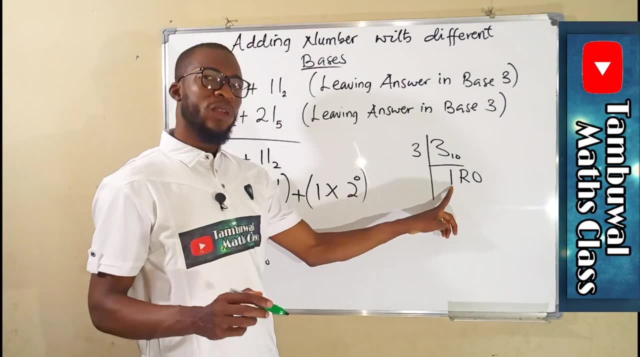 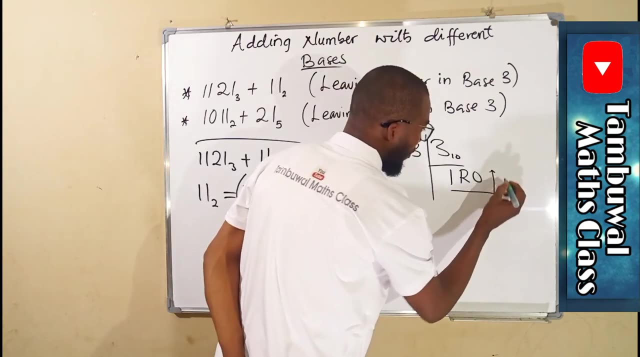 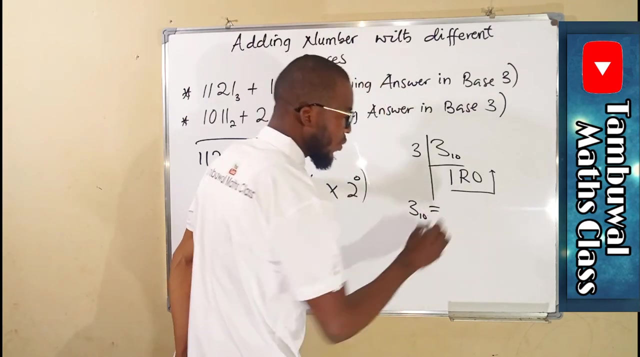 From 3 you can go to 3, 1 time without remainder. There is no remainder. 3 can no longer go into 1.. So we stop and take the number from this other 1 and forward. Thus we see 3 in base 10 is equal to 1, mean 0, in. 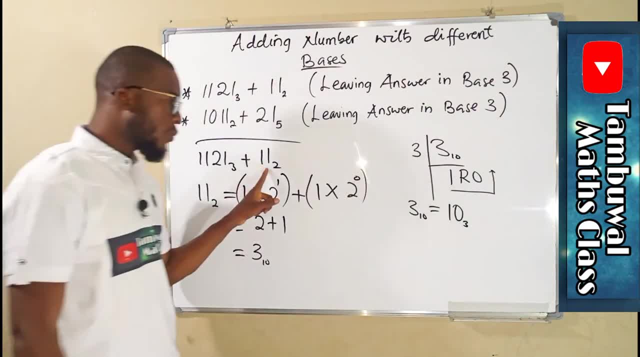 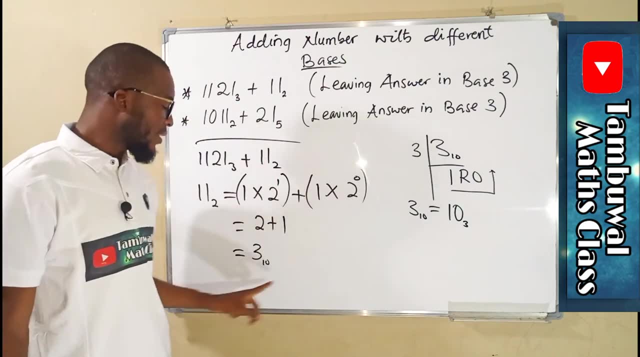 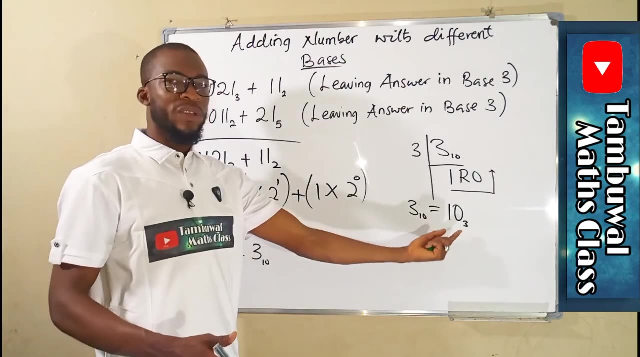 base 3.. means that 1- 1 in base 2 is exactly the same as 1- 0 in base 3, because we use this to convert it into base 3. they are the same, just that they have different bases and we use this to convert it into base 3. so these three numbers, 1- 1 in. 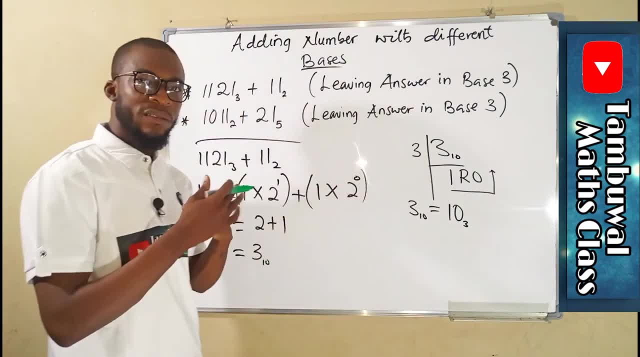 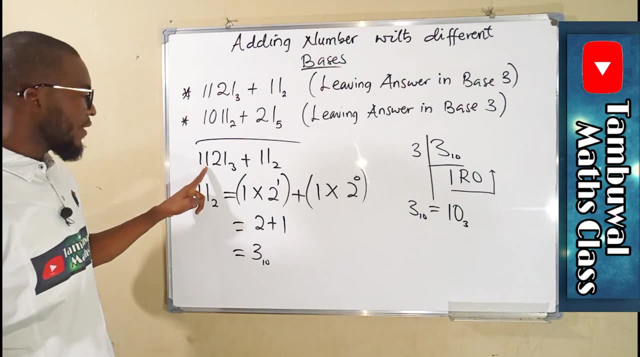 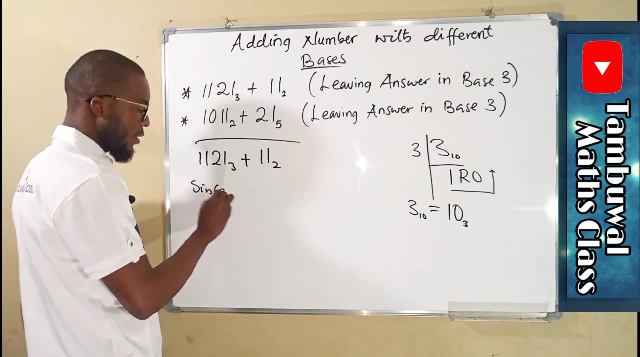 base 2, 3 in base 10 and 1: 0 in base 3. they are exactly the same, just that they have different bases. so now we are free to add this number and this number together, since 11 in base 2 is equal to 10 in base 3. now we can say this plus: 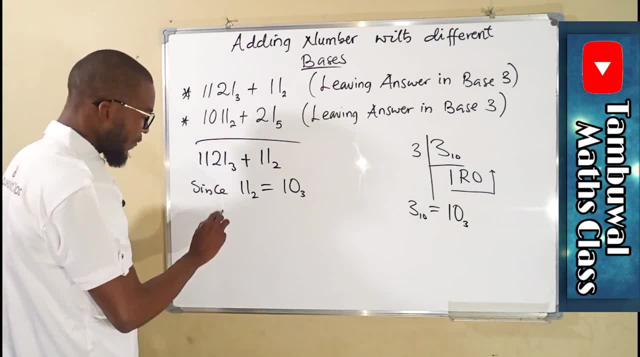 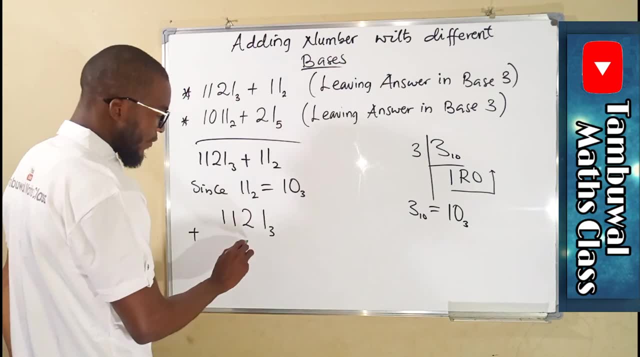 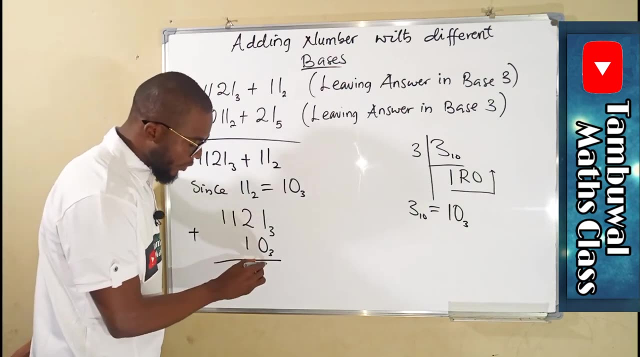 this is the same thing as this plus this. so we have one 1, 2, 1 in base 3, plus we have 1, 0 in base 3. we then add together: 1 plus 0 is 1. 1 is less than the base. 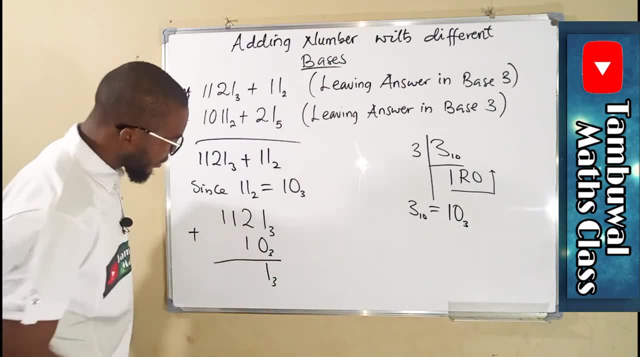 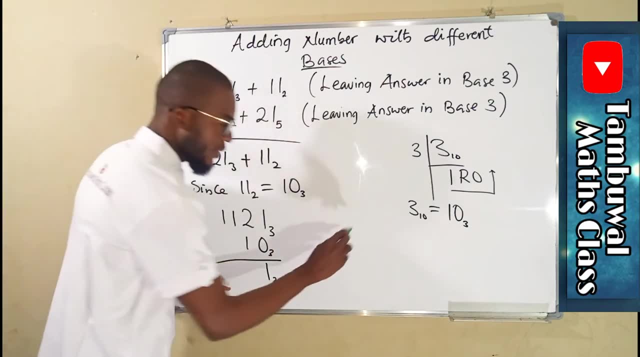 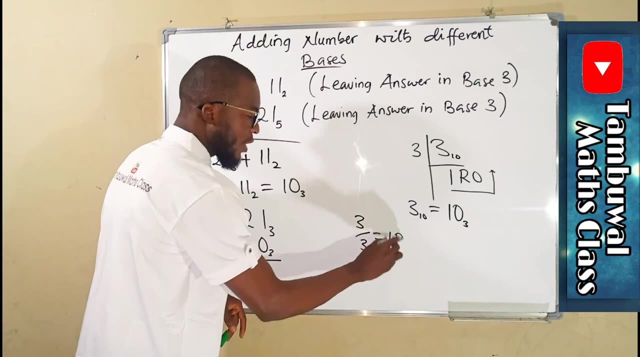 so we can write it. this is base 3. 2 plus 1 is 3. 3 is exactly as our base. so we take the remainder. we say 3 divide by the base, which is also 3. 3 can go into 3 one time without remainder. 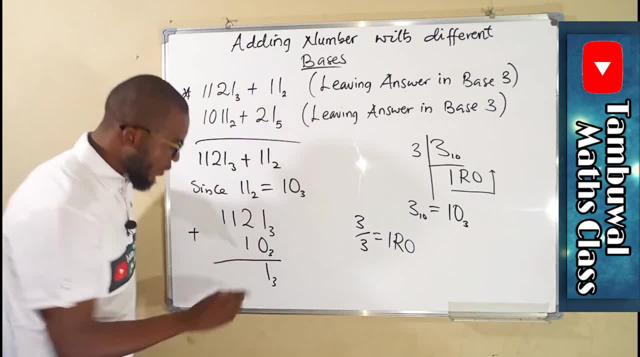 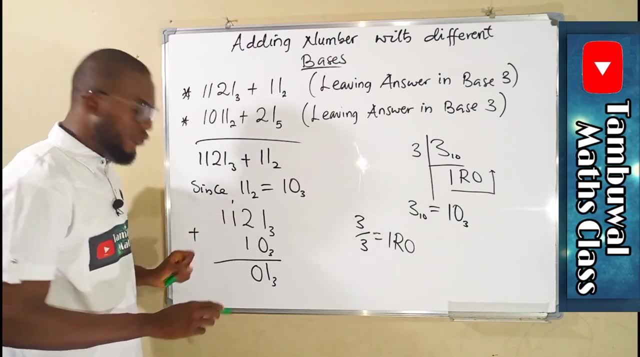 so we write the remainder, which is 0. then we take this 1 to the next level. we have 1 plus 1 is 2. 2 is less than the base, so we can write it. and finally we have 1 plus nothing is still 1. 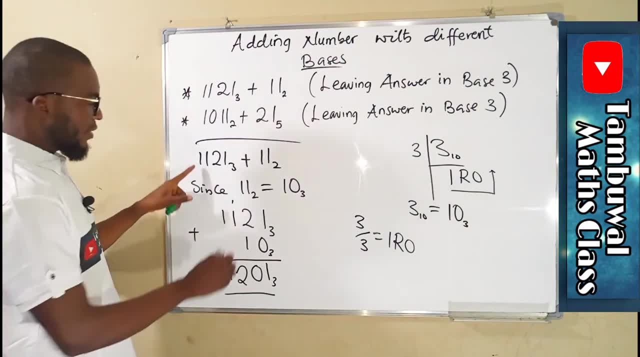 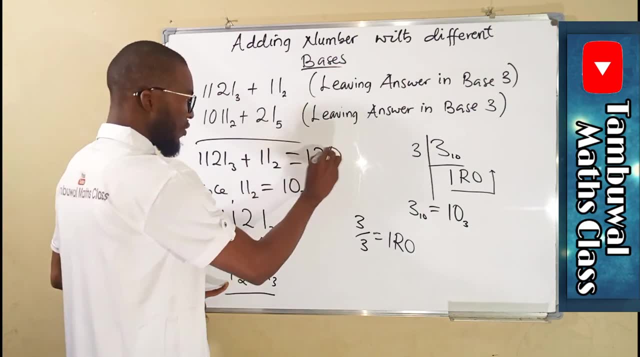 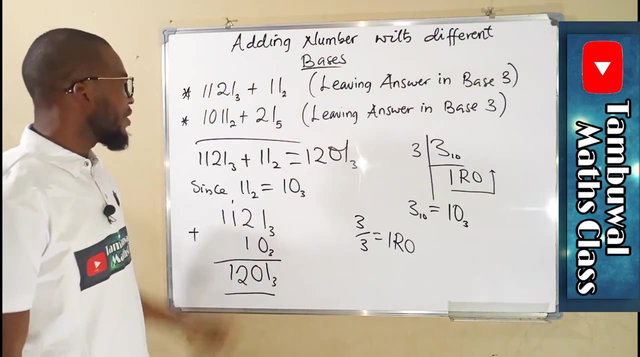 so finally, you can see that this plus this will give us 1,, 2, 0, 1 in base 3. because this is 0, say we should leave the answer in base 3. now let us look on to the next question. 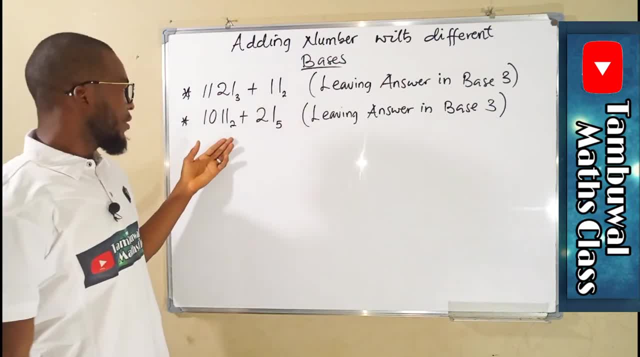 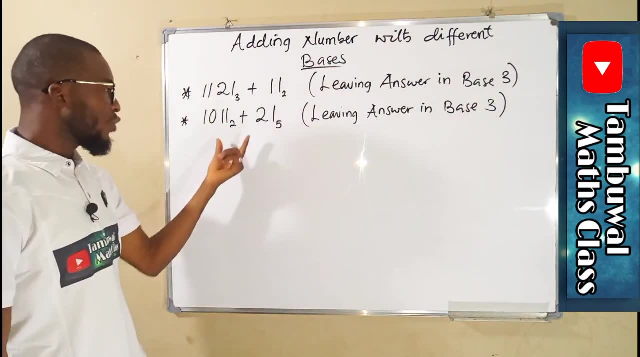 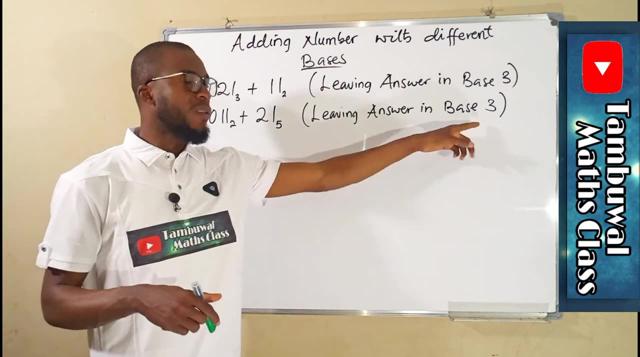 which is this. in the second question you can see, none of the numbers is in base 3, so now we are free to convert each of these numbers into base 10. then we add the results together, then we re-convert the result into base 3 and we are good. 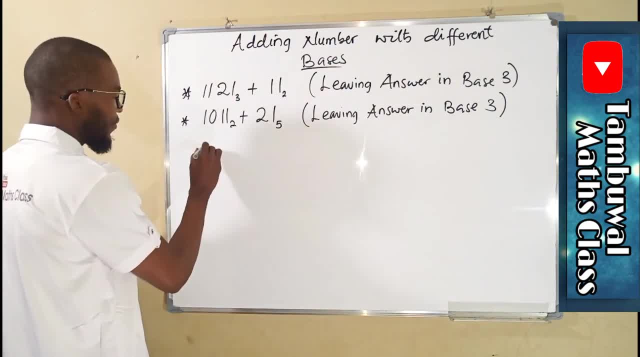 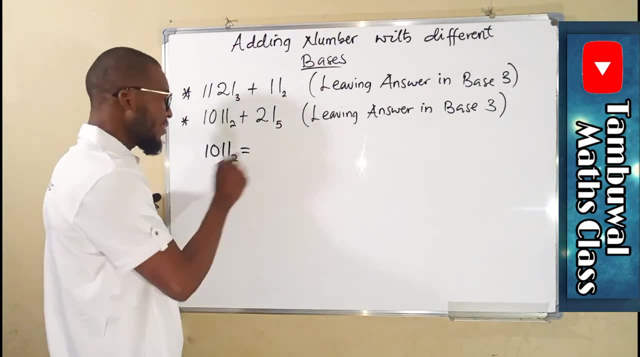 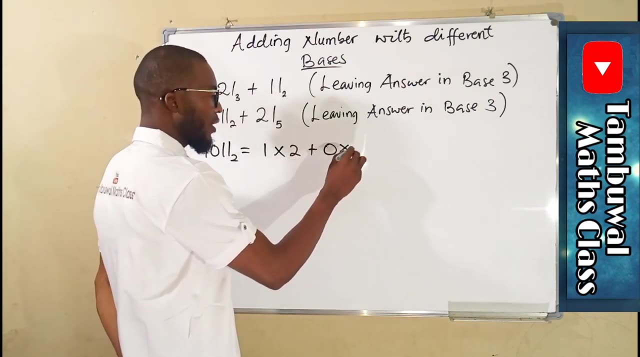 to go. let's start with this one. we have 1, 0, 1, 1 base 2. we want to change it to base 10. we take the first digit, 1, we multiply by the base 2, we add. we take the second digit, 0, we multiply by the base, which is 2. we have 1 times 2 plus. 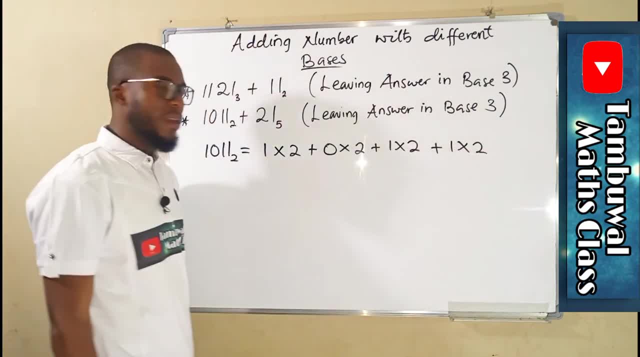 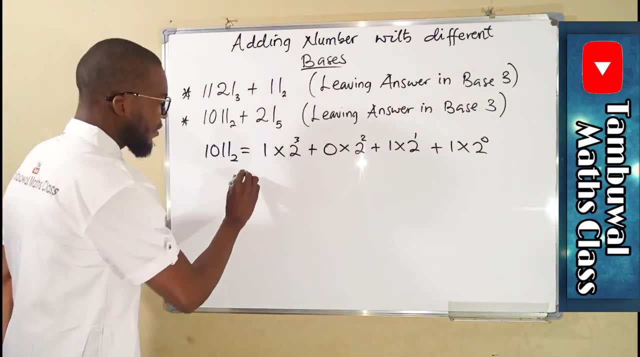 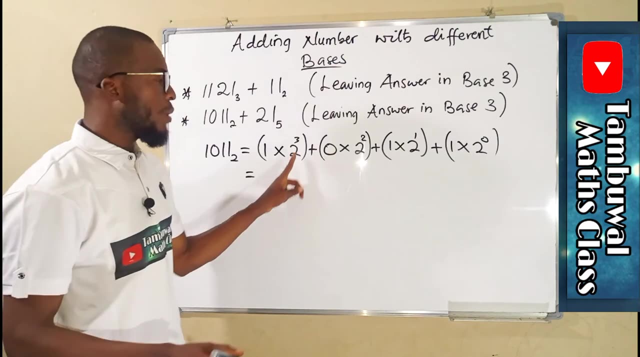 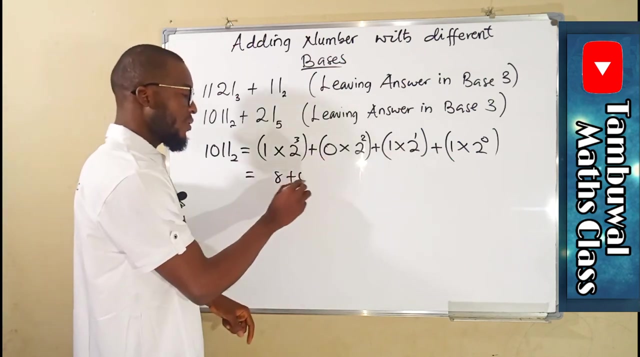 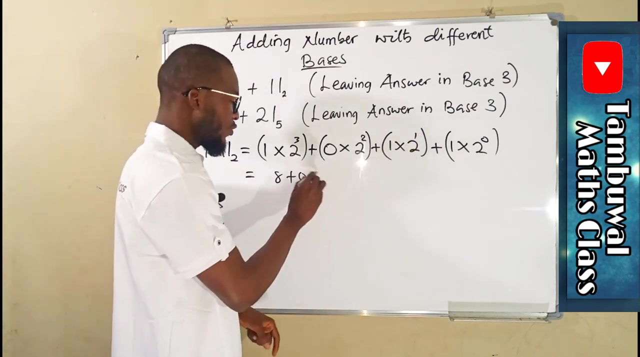 the last one, 1 times 2. we assign our index from the right to left: 0, 1, 2, 3. we stop. we simplify: 2 power 3 is 8, 8 times 1 is 8. we add this time this is 0, because 0 times 4 is 0: 2 power. 1 is 2 times 1 is also 2: 2 power. 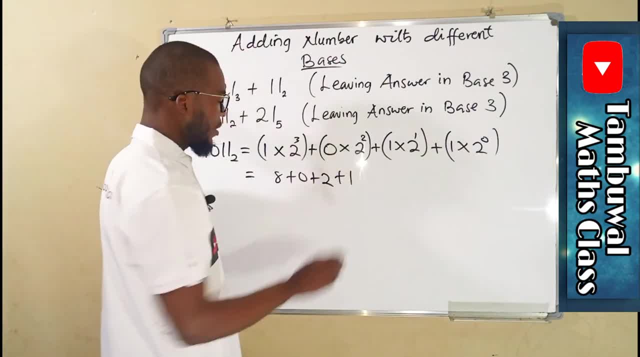 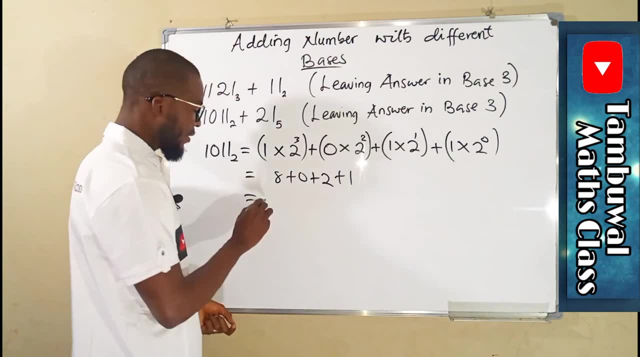 0 is 1 and 1 times 2.. one is also one. then we add all of this together, we have eight plus zero is eight. eight plus two is ten plus one is eleven. this eleven is in base ten. now let us take the other number, which is: 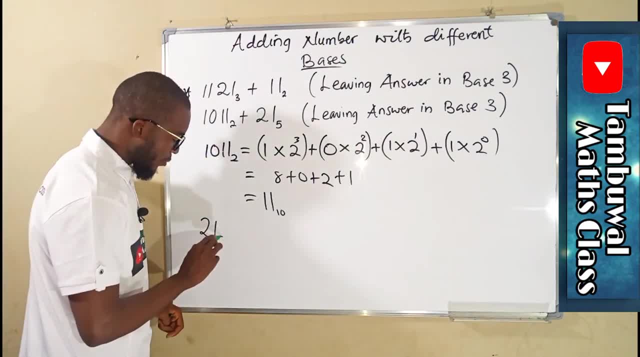 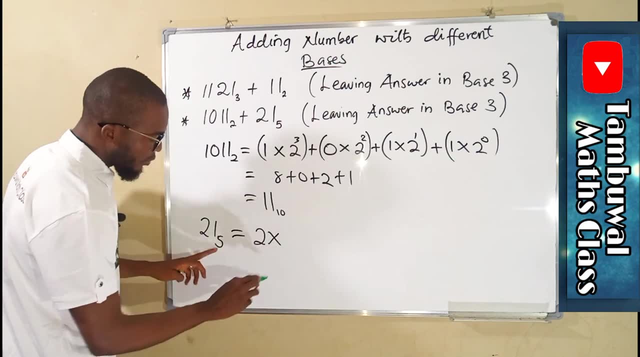 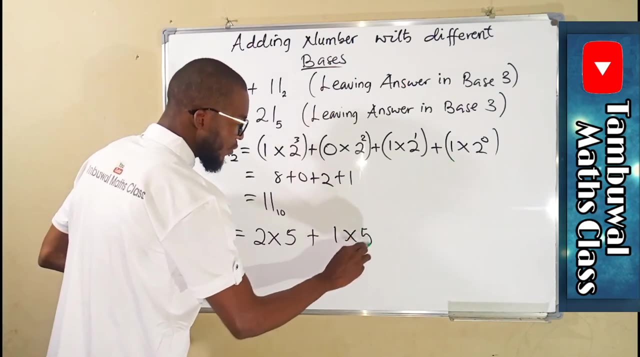 twenty one in base five. twenty one base five. we convert it to base ten as well. we take the first digit two, we multiply it with the base, which is five, we add. we take the second digit one, we multiply it with the base, which is also five. we assign our index from right to left, starting from: 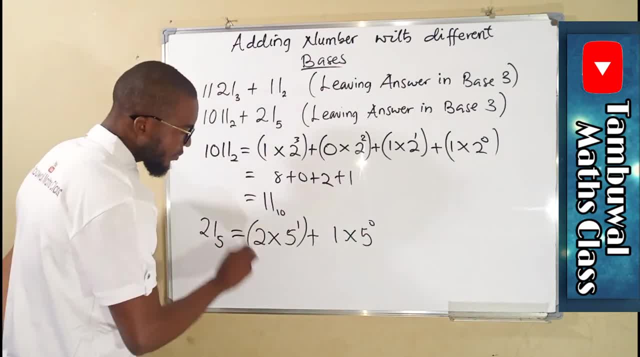 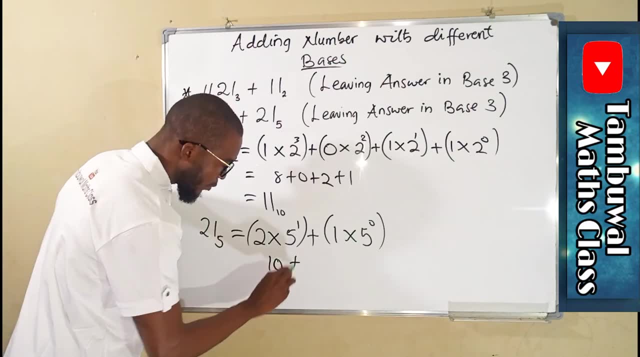 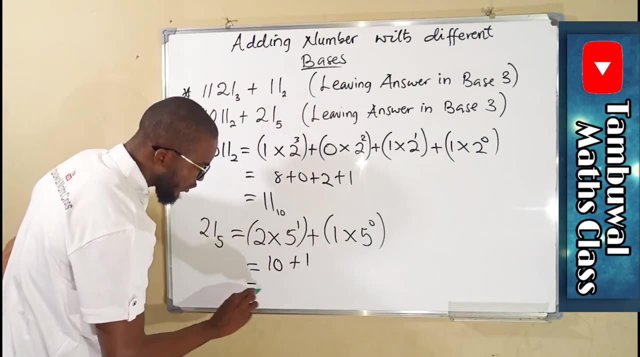 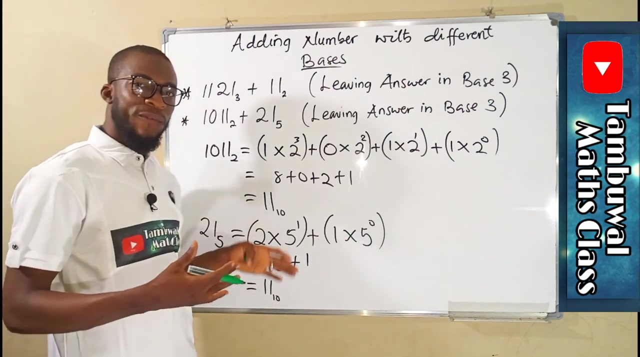 zero one, we stop five. power one is five times two is ten plus five. power zero is one times one is also one. so this is also eleven in base ten. now, since we have converted all the two numbers into base 10, we are free to add the base 10.